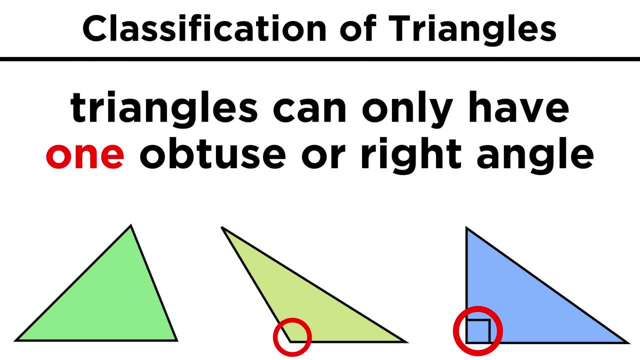 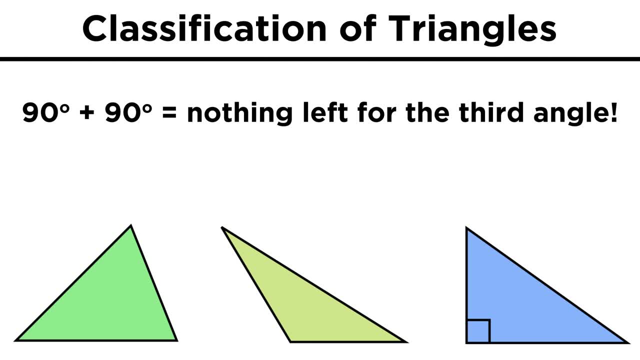 This is why any triangle can have at most one right or obtuse angle, because two of them would add up to one hundred eighty or more, and then there is nothing left for the third angle. This fact will help us algebraically determine the measures of certain angles later. 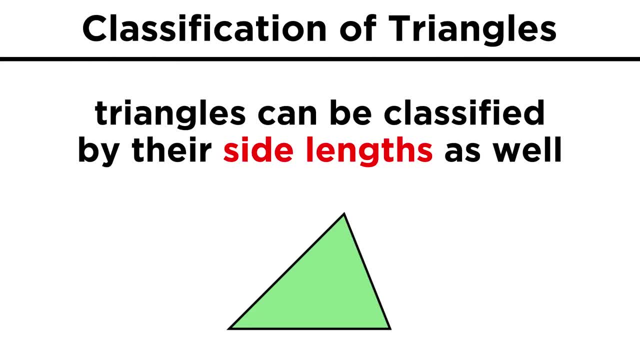 Triangles can be divided into two parts. The first part is the right angle and the second part is the left angle. Triangles can be divided into two parts. Triangles can be classified not just by angles, but also by side lengths. 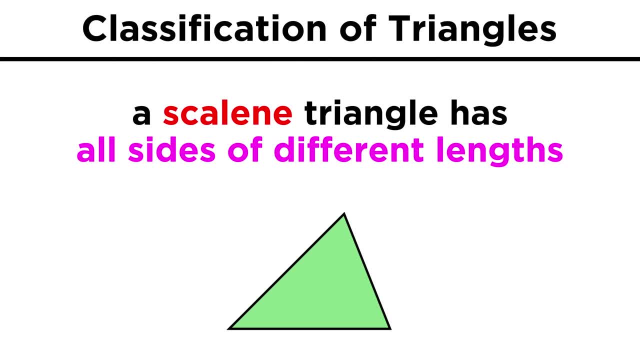 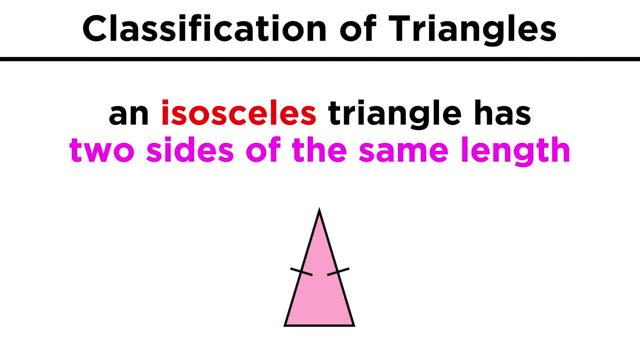 A scalene triangle is defined as having three sides of different lengths. An isosceles triangle has two sides out of the three that are exactly the same length and therefore two angles that are precisely the same measure, specifically the two angles that are opposite, the two identical sides. 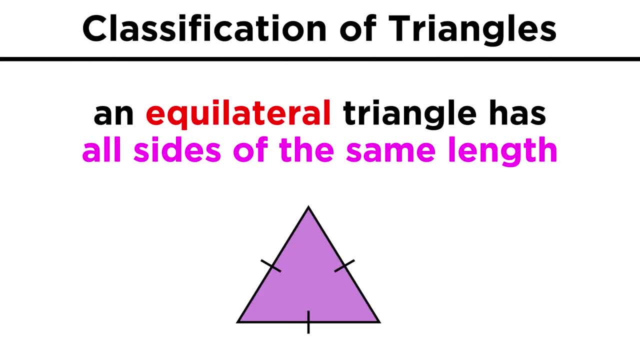 And an equilateral triangle has all three sides of the same length and therefore the three identical angles. Since the three identical angles must add up to one hundred eighty degrees, each angle must therefore be sixty degrees in an equilateral triangle. Every triangle must be one of these three types because if they have three sides, it. 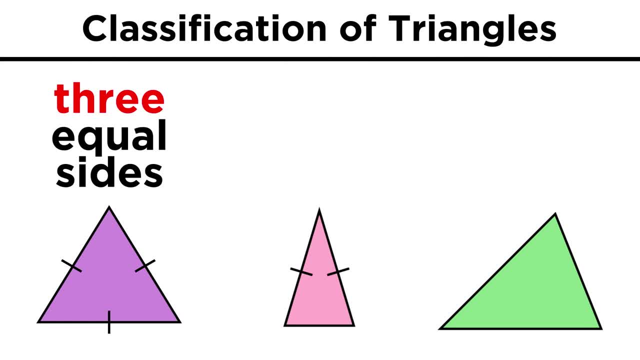 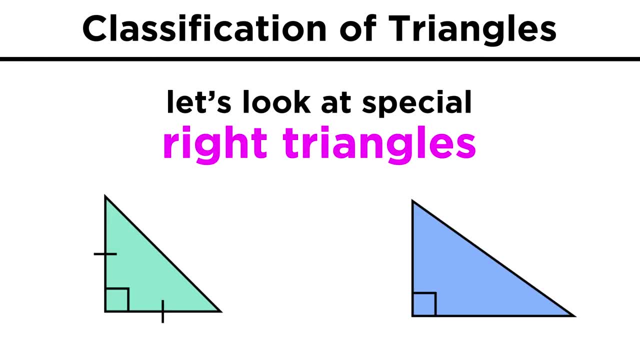 must either be the case that they are all the same, two are the same or none are the same. as those are all the options we have, It's worth our time to also quickly mention some special kinds of right triangles. One is the forty-five, forty-five, ninety triangle. 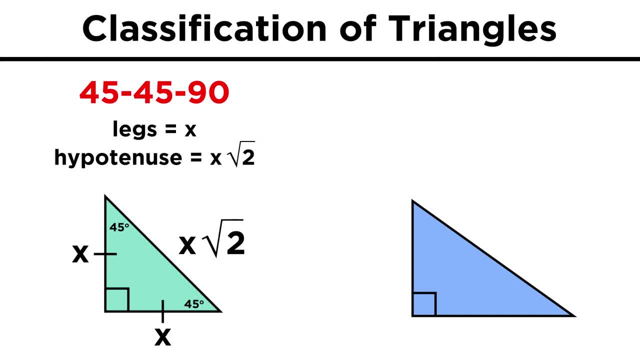 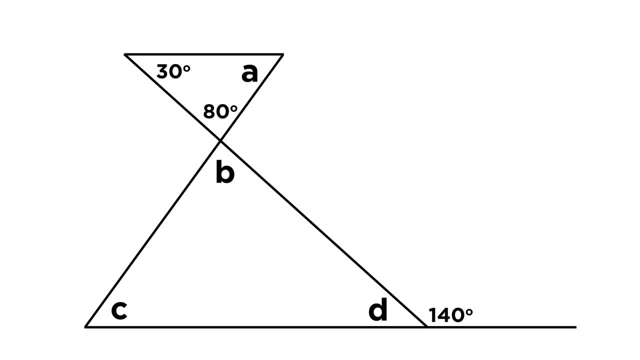 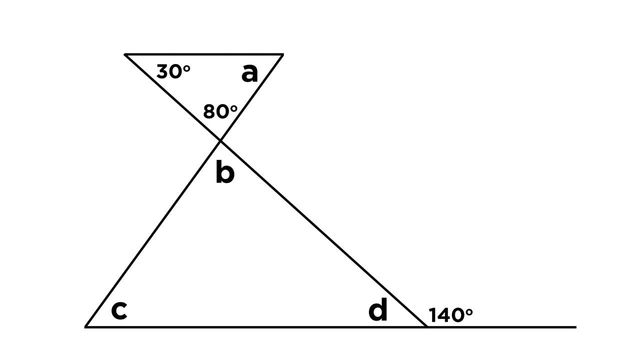 We just fill them in one at a time. by using the rules we know, If we have one of two vertical angles, the other will be the same as the first. If we have two angles in a triangle, then the third will be one eighty minus the other.